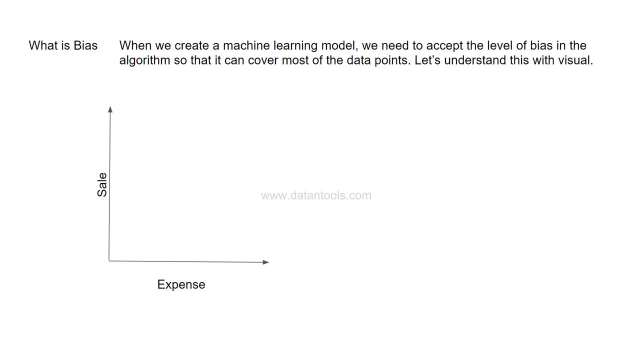 sale. on the x-axis you have expense. so expense is nothing but the marketing expense and generally the assumption is that if you have more marketing expense you have the higher sales numbers. so these are the data points, which represents the same assumption. Now, if we need to identify what will be the sale at a particular level of marketing expense or a, 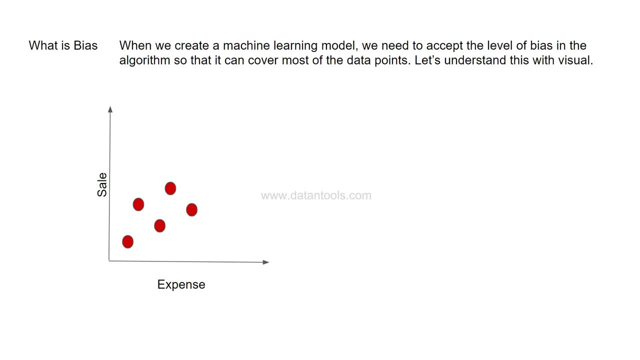 particular point of marketing expense. we need to fit an algorithm so that we can do the prediction. Now, since these lines or these data points represents the linear trend, it is a good candidate for linear equation or a OLS, which is ordinary least square method. Now to fit it. what I will show you is basically some comparison. 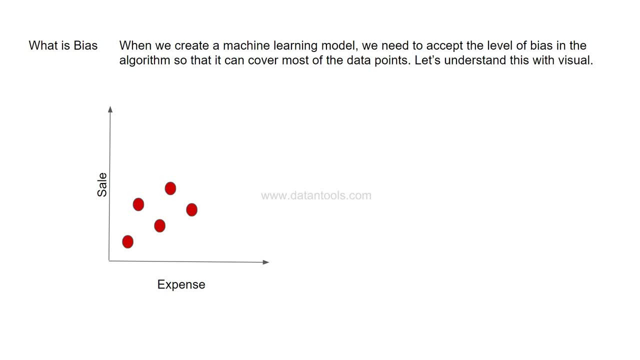 between the line to help us understand the bias Now, whether this line represents truly represents all the data points, or this line truly represents all the data points, or this line truly represents the data points. Pause the video for a minute and just try to understand this chart. So I hope by now you have understood this chart, but if not, what we are. 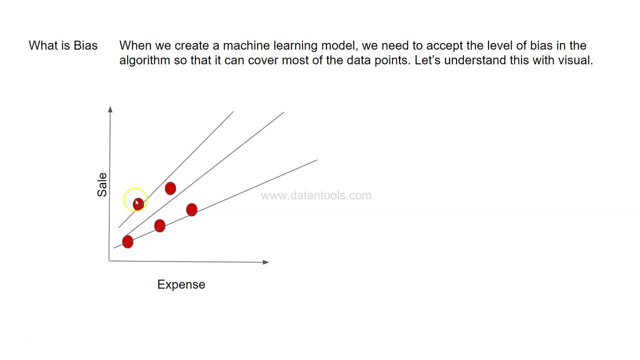 really trying to understand over here is that we have these five different data points and we need to figure it out which line is best representing all these five data points. and by now you must have figured it out by looking at visually that the line here in the center is representing is 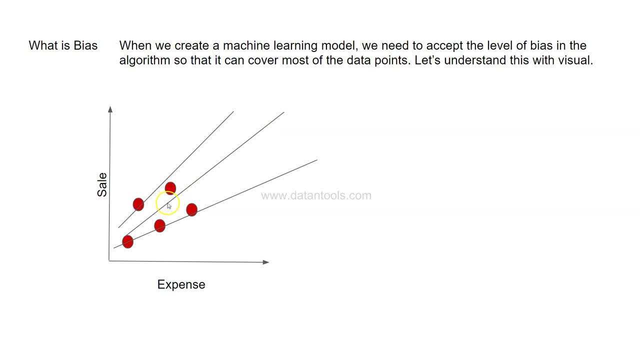 best. Why? because from this line, the distance between each of the data points is less, For example, if you have only this line. so if I just go to step back, if I only have this line, the distance from this line to this data point is high. this data point, distance from this data point is high. 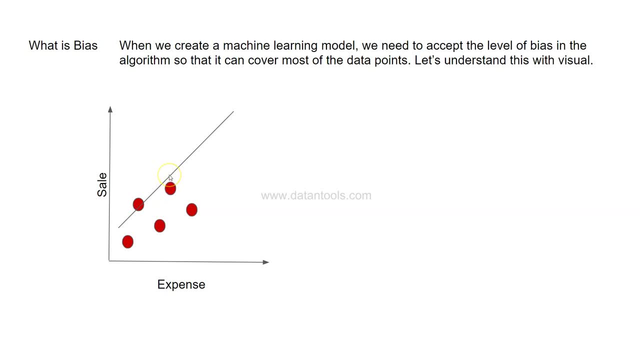 distance from line to this data point is low and, finally, the distance from this line to this data point is high. So it is. so there are a lot of data points, for example these three data points, which are relatively far from the line. Now, if I let's say, if we have tuned the parameters and 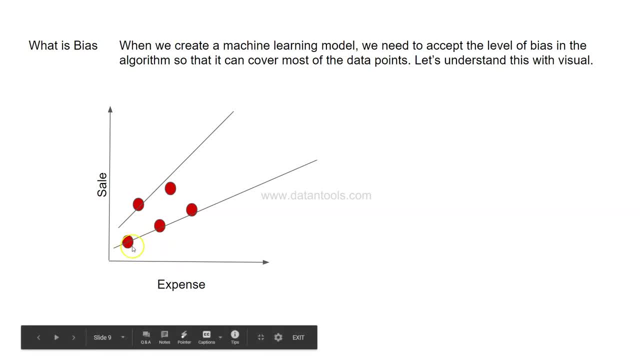 created a new model which is say: seeing that, based on these three data points that you have available, the new function is fitting the line like this. but even in this case we have the, we have some of the data points which are very far from this line. Now again, we further tune the parameter values or 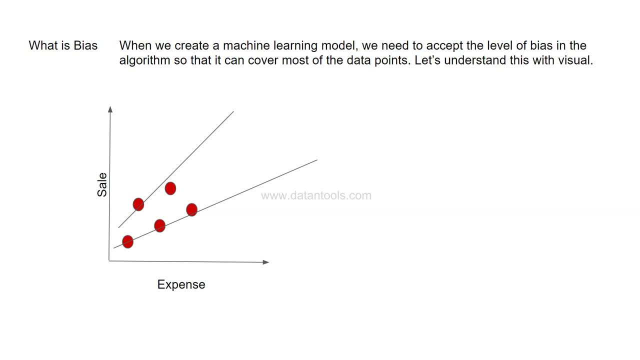 we further fit the the model on the training data and we figured it out that this line is the new line which is reducing the distance between the data points. and finally we say, yeah, this line really represents, or truly represents, all the data points. Now, this is basically what we call is. 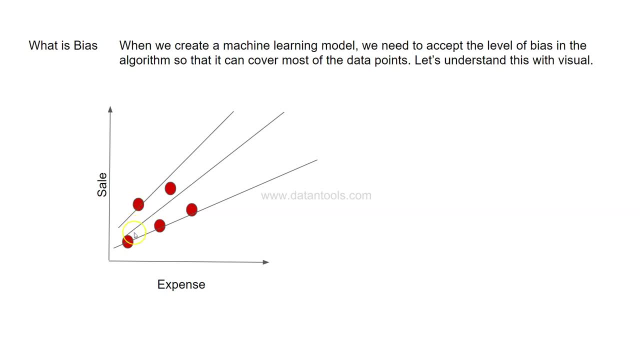 basically a bias. So bias is nothing. but you know, you have these, all these distances from the line, and we need to reduce the bias by having the best fit line or the best fit model, which is having the representation of all the data points with the minimum bias. All right, 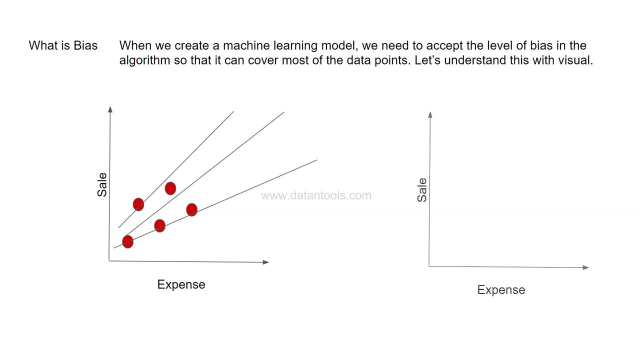 now, apart from this, one can even have a model like this. So what do we have is basically a non-linear model. You can use the non-linear, nearly non-linear- what I want to say- non-linear function or non-linear modeling approaches which will try to fit all of these data points all very perfectly. But this is something which is called 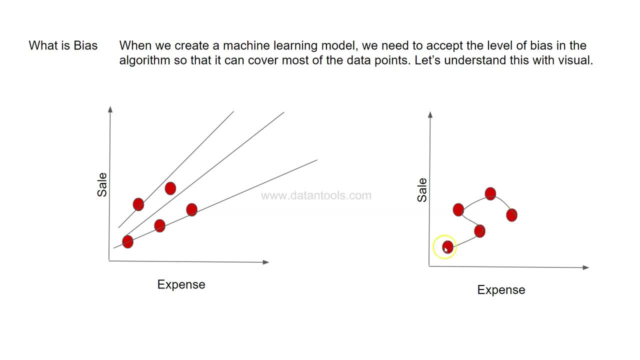 as overfitting, and the reason for this is that, though, it will work well when it comes to training the data. So this is something which is called as overfitting, and the reason for this is that, though, it will work well when it comes to training the data. 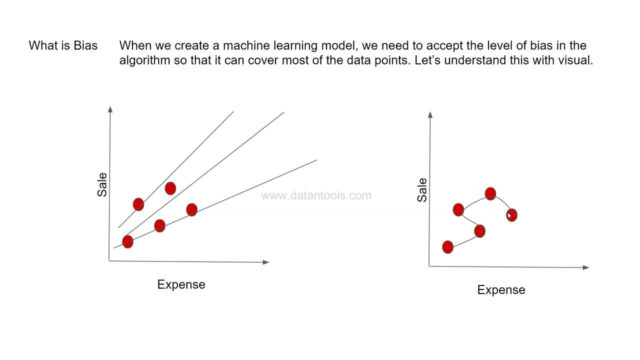 But when it will see the new data points to make the prediction, it performs very bad. So we try to avoid the situation where we are trying to learn each and every data point from the training data very accurately. In that way, you are having a very high influence of training data on your model, which may not result into a good prediction. 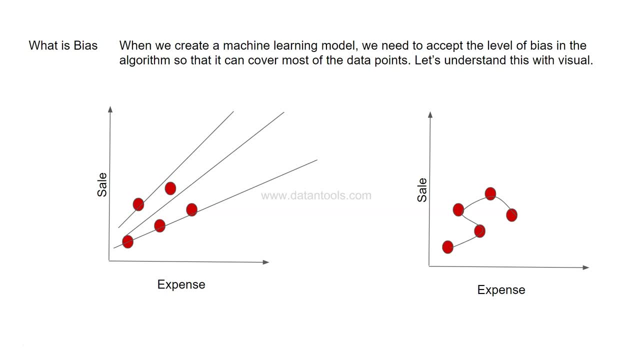 on the unseen or the test data. So let us go ahead and now understand the variants. So what is variants? Variants is nothing but the difference between the fit of training and testing set. So let us say: what I have over here is basically what I showed in the previous slide, the BEST model, which 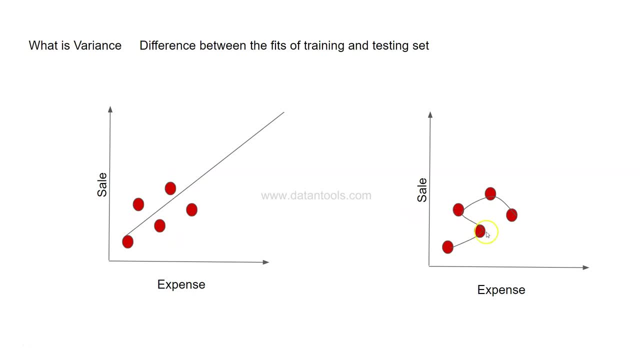 is representing the data points, And then this overfitting model which is trying to then in the former model, which is trying to calculate onlyята models within the data point of fence two horizon, and then this overfitted model over here is basically the what I showed on the previous slide, the best model, And then this overall fitter model. So for the purpose is, 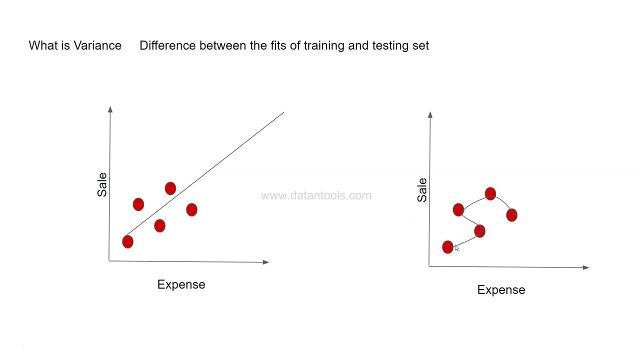 to capture most out of the training points and let's see how well they fare on the unseen data or the testing data. so what do we have is basically these three data points, which is the testing data points, and over here, from this line, you can see that there is. this line will do a better job in terms of predicting. 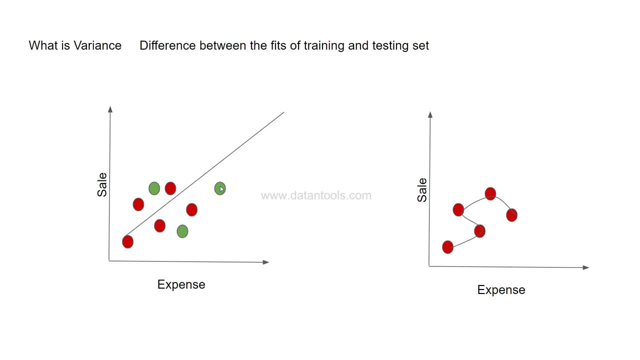 it and after the prediction, it has plotted the data points over here and then we calculate the variance for these three data points. now, if you have the same data points over here, you will see that in one of this odd cases it will work fine. but if you see this data point, this in this case, the distance is pretty. 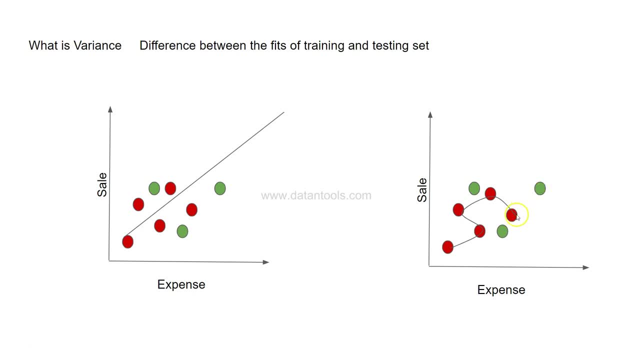 high, and same is the case with this. in this case, the distance will be pretty high, so that's why this overfitting method or this overfitting technique will not going to work in more than one case. so when you are looking at most of the scenarios where you know you have 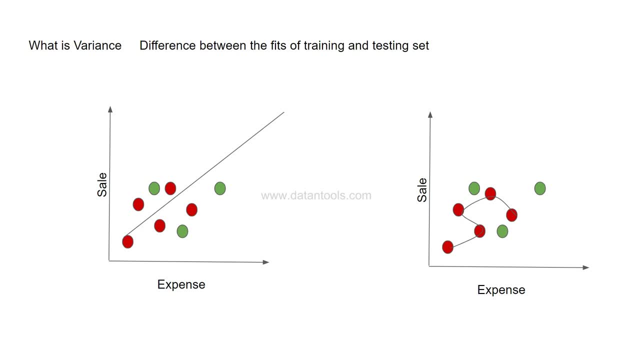 almost negligible variance. there has to be some variance- sorry, some bias- which is a true representation of all the data points, and we should accept that bias so that whenever we are showing the unseen data points, like these three green data points, then our model should be able to predict and have the low variance, even in. 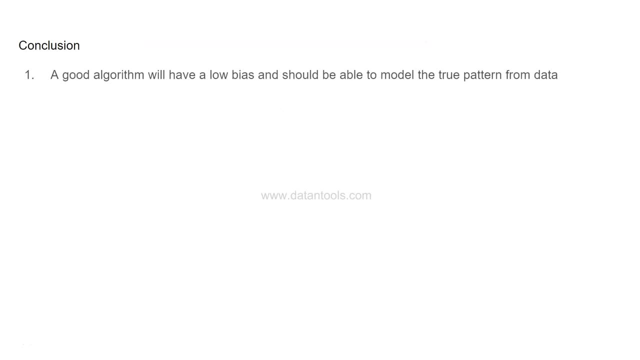 that case as well. finally, what is the conclusion? conclusion is that a good algorithm will have a low bias and should be able to model the true pattern from data. algorithm should be able to predict the new values consistently with low variability. that means the low variance, so your algorithm should have low.